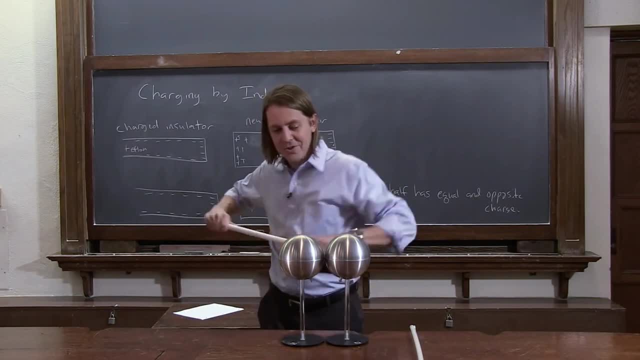 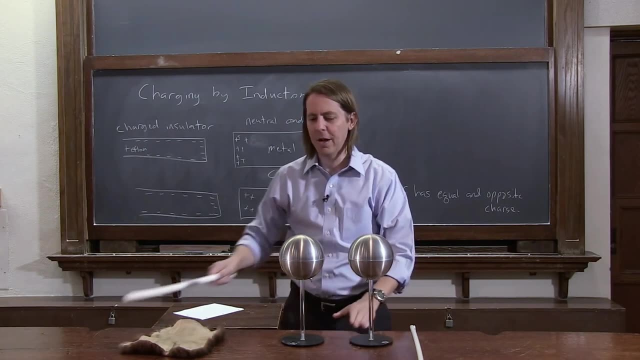 You didn't see anything. Well, there's nothing to see. So let me charge it up again. Bring it over here, And now I'm going to cut, I'm going to separate them, And now we just charge the two spheres by induction. 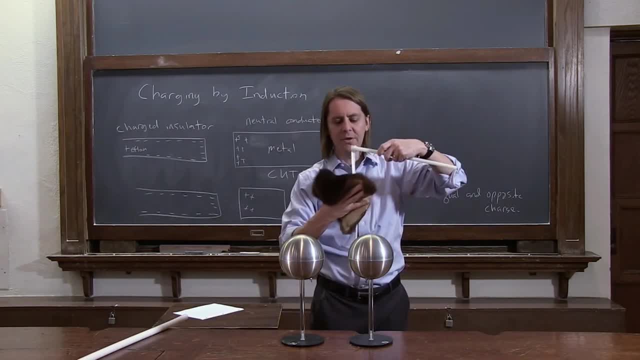 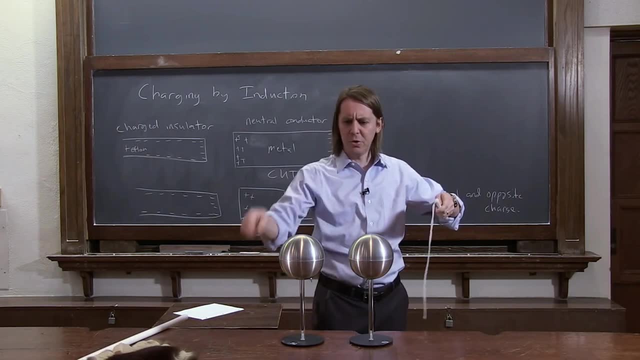 Of course you can't see it. I'm going to try to prove it to you with a little bit of Teflon tape. So we know, if we rub fur on this Teflon tape, we know it ends up negative. So if this 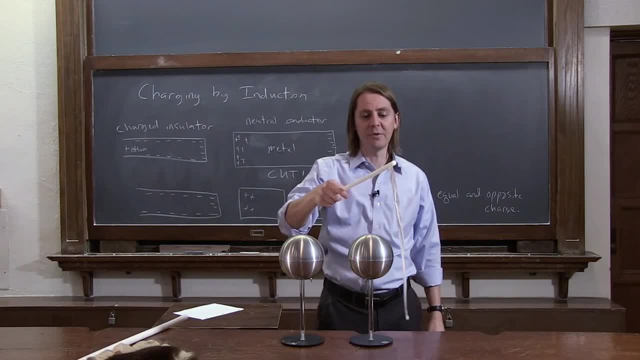 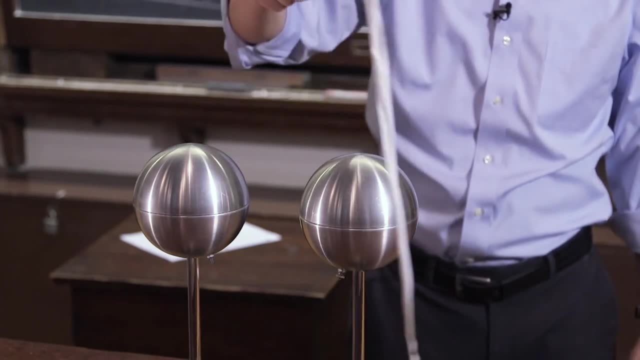 thing ends up negative, then they should repel each other, or the tape should be repelled, And sure enough. you can see the tape is repelled. It doesn't want to touch the metal. And we should have left the other one positive, And sure enough. 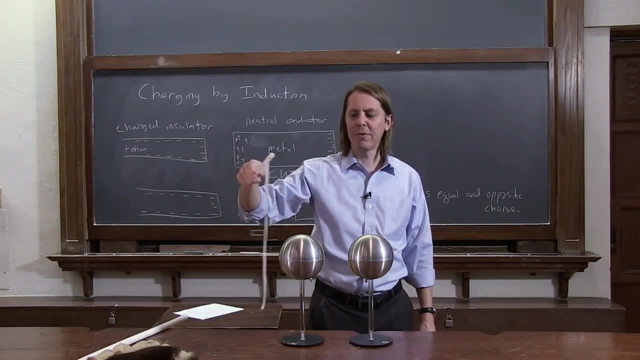 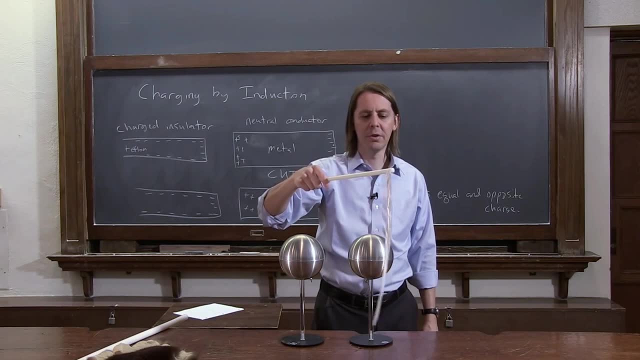 it's positive. It's very sticky for the tape, So I'm going to use a Teflon rod or a Teflon tape to confirm it really did what it was supposed to do: Repulsion there. There's one other way we can confirm it: It's when I bring them together. 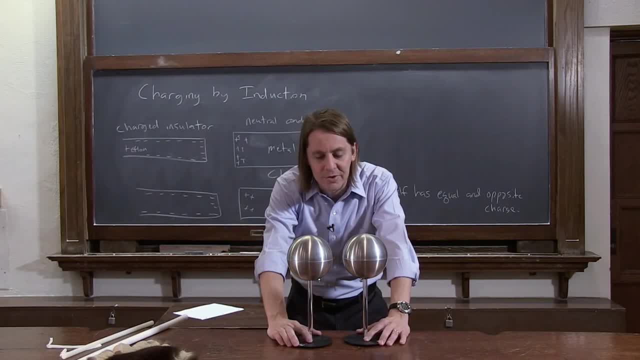 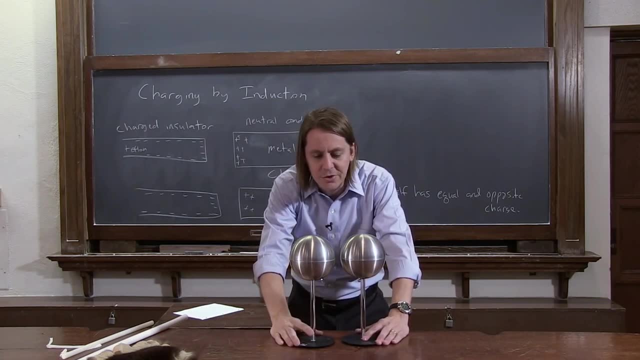 If you look very close, you can see a spark jump across the gap. The negative charge, the positive charge comes back together, makes a corona and an arc, like we talked about before, And you can actually see the charge go back. So seeing is believing. 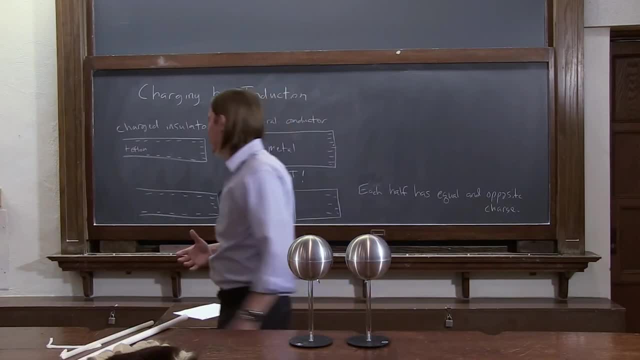 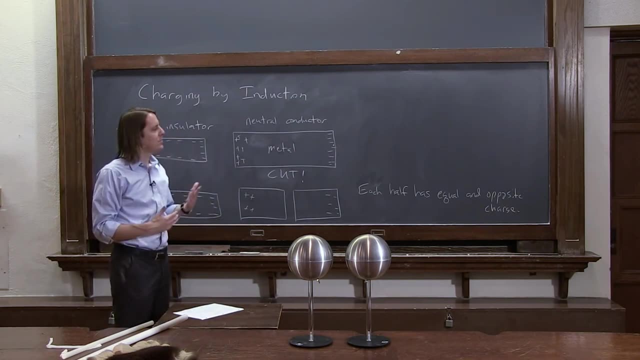 And there it was Okay. So charging by induction It's also not a quantitative thing like rubbing. We aren't going to calculate the amount of charge that we pushed around. Maybe we can do that later, But for now it's just another way to think about how charge behaves in a material.